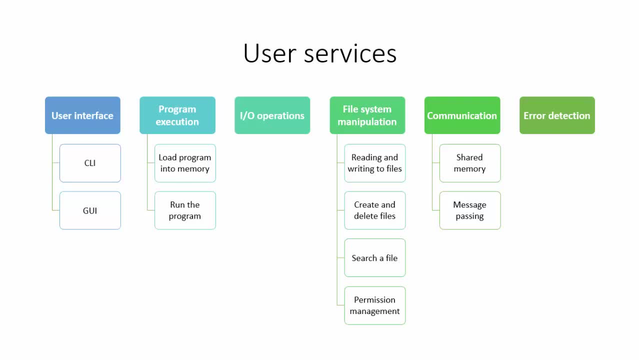 All that is available is the keyboard And the screen. For anything to do, you need to remember a command. For example, if you want to create a file in command line interface, there will be a command for this, But in a graphical interface what you can do is you can simply right click new and then you can create a file. 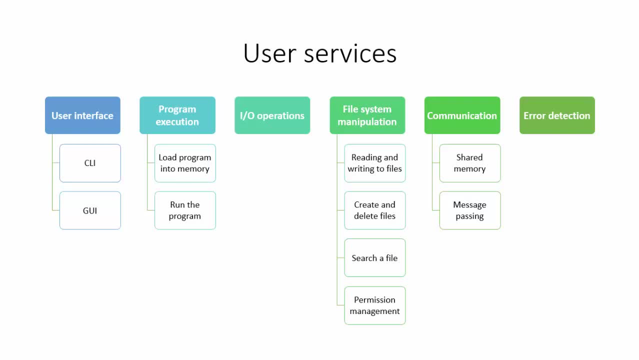 So both these command line interface and graphical user interface has got their advantages and their own disadvantages. The graphical user interface is very easy to learn, But the power of the command line interface is more as compared to the graphical user interface. Command line interface is very difficult to learn in the beginning. 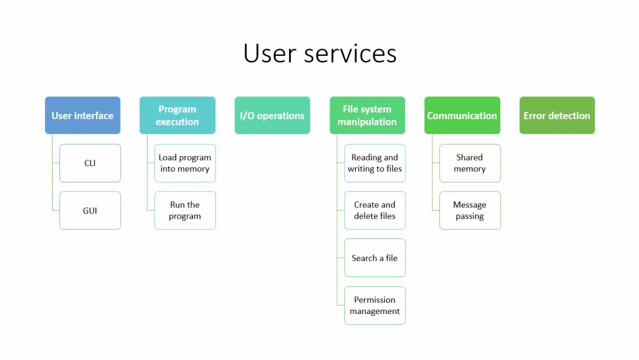 So I will give you a small example. If you want to create a file in graphical user interface, it is very easy: Right click new and you create a file. But with command line interface you need to know what is the right command to create a file. 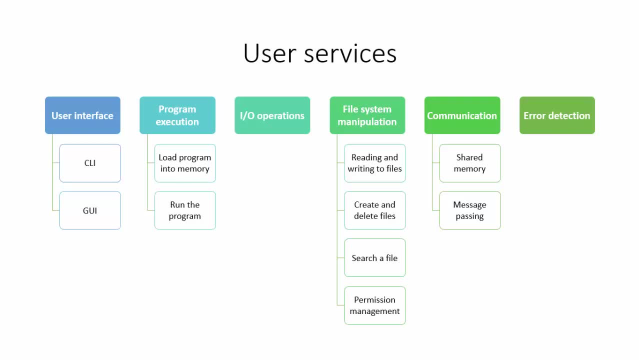 And that command might differ from one operating system to another operating system. Now, what are the advantages of command line interface? Now, what are the advantages of command line interface If you want to create, let us suppose, 1000 files with the names 1 to 1000.? 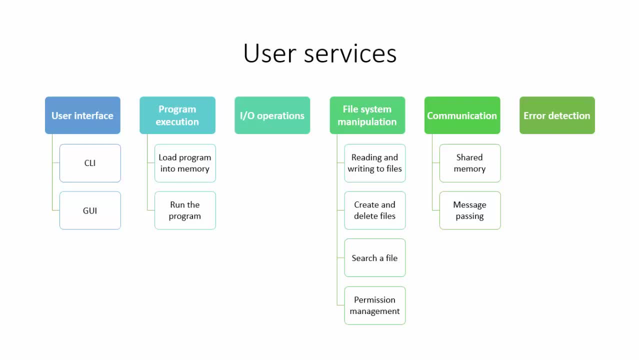 Now just think of how much time it will take. in the graphical user interface, Right click new and then you give the file name Again, right click new and the file name and so on. Right, I think, even if you try on your best, the best of your speeds, you can do it in 10 minutes or 1 hour. 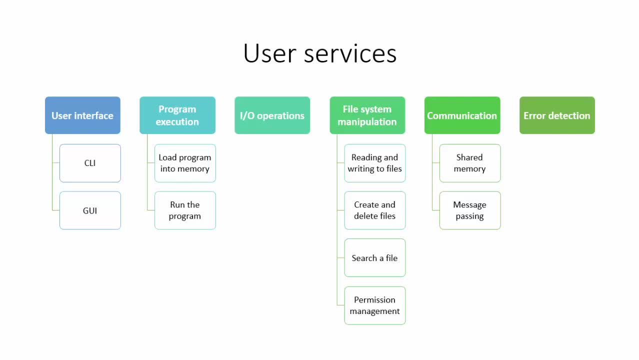 But with the command line interface, if I take an example of Linux, the command is going to be touch and then 1, dot, dot, 1000.. That's it. So with the right command, you will be able to do a complex task in the least amount of time. 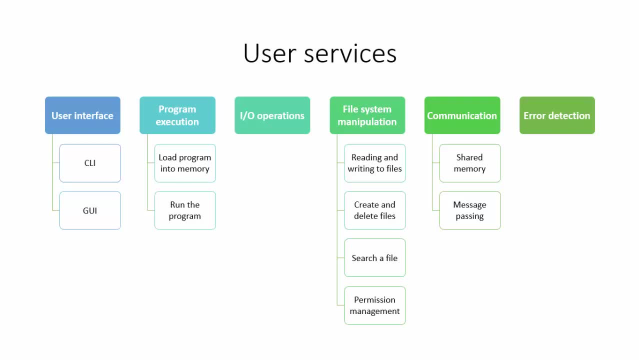 Now coming on to the second service program, execution. So the operating system has to take care of how to load a program in the memory, How to load a program in the memory, where to place it in the memory and how to run the program. 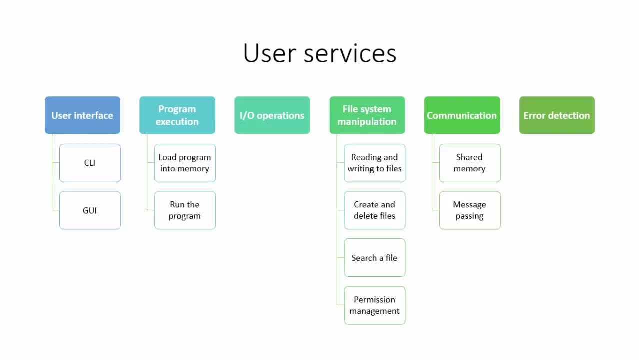 For the user. it simply has to be a double click. So whenever you want to run a program- let us suppose MS Word- what do you do? You simply double click on the icon of MS Word and it starts. What happens behind? how that Microsoft Word is loaded into the RAM, how it runs, that is to be handled by the operating system. 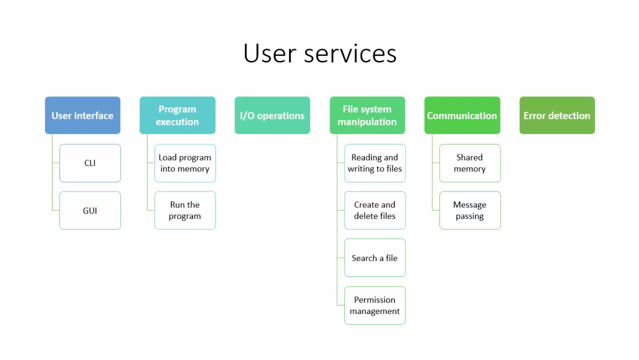 The third service is input output operations. So during the execution of a process, the process is required to take input from the user or it might want to give some output to the user on the screen or on the printer. Now, how to handle those input or output devices? 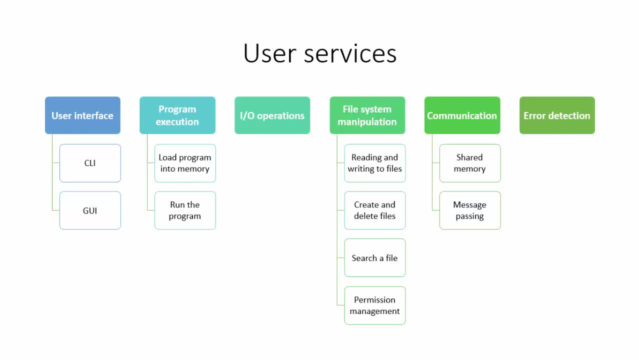 All this will be done by another service, that is, for all the input output operations, So that the user don't have to bother how a keyboard works or how a printer works. Everything will be taken care by the operating system. The fourth service is file system manipulation. 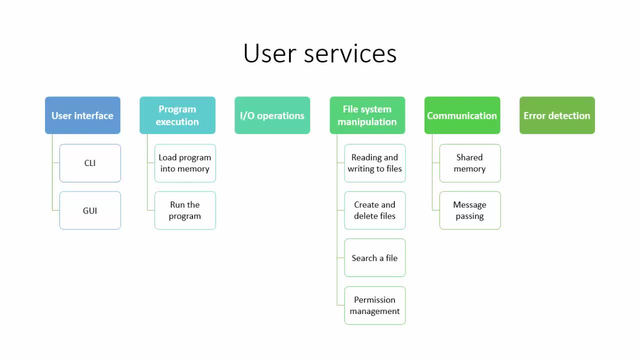 So, whenever you want to manipulate a file, manipulation means you want to read the file, you want to write into a file, you want to create a new file, search into a file, anything. We never bother whether we are allowed to do it or not. 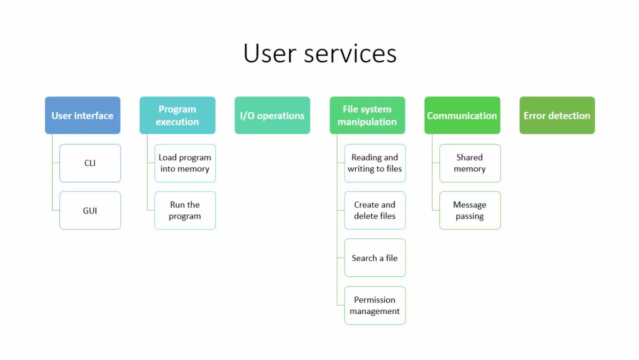 The system takes care of this. For example, you open a file Now, as a user, are you allowed to open that file? This will be taken care by the operating system. Are you allowed to write into that file? This will be taken care by the operating system. 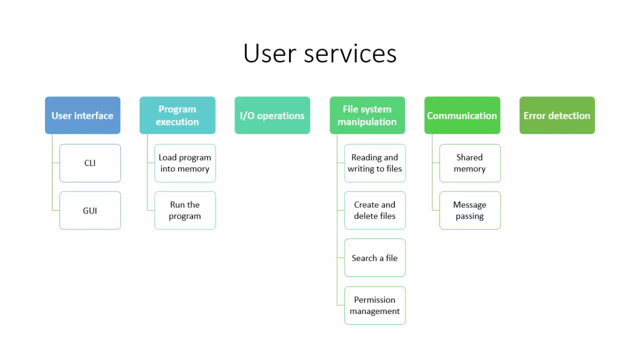 How to store that file. That file needs 10 MB space. Now to find that 10 MB space in the hard disk, that is the job of the operating system. The fifth service is communication. Sometimes two process might want to communicate. They might want to send some message to one another. 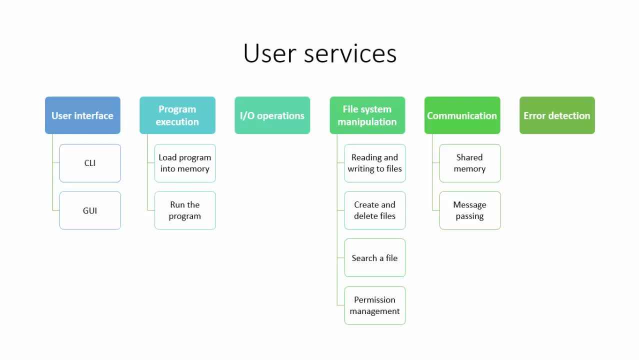 Now those processes might be on the same system, They might be running on different systems. So to send a message from one process to another process, the entire procedure has to be handled by the operating system. So to send a message from one process to another process, the entire procedure has to be handled by the operating system. 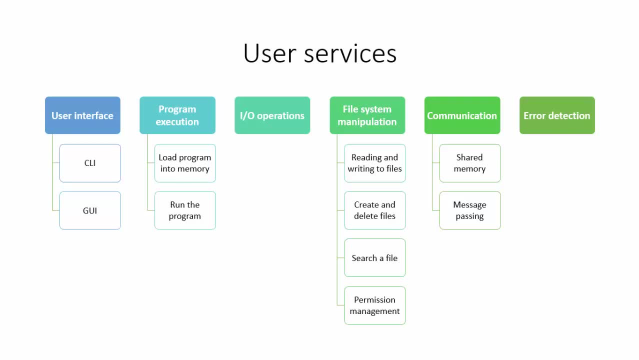 This communication can be done in two ways, Either by using shared memory or by using message passing techniques. So this we are going to discuss in detail in another topic that will do on inter-process communication. The last service to the user is error detection. 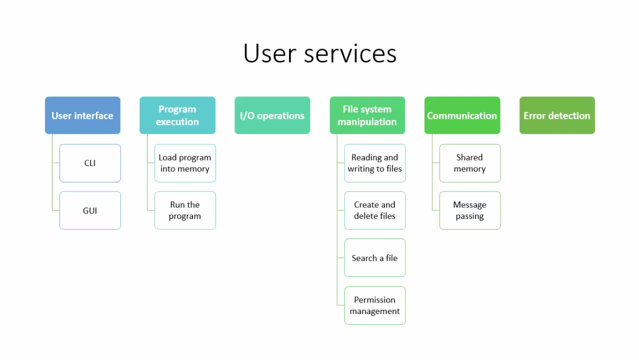 Whenever this operating system detects some error in the system, it should report it to the user So that the user can take an appropriate action on that. So error detection is a very important part And certain times the OS might have the capability to automatically debug the program or debug that error that it has detected. 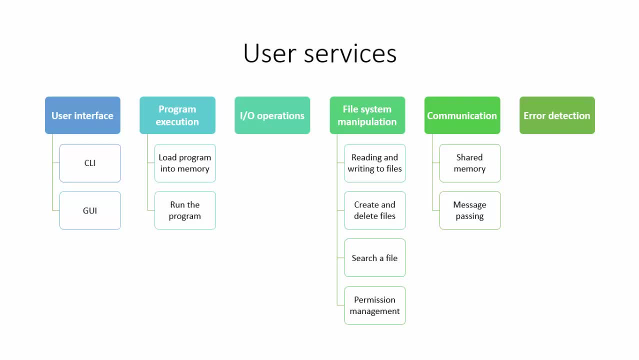 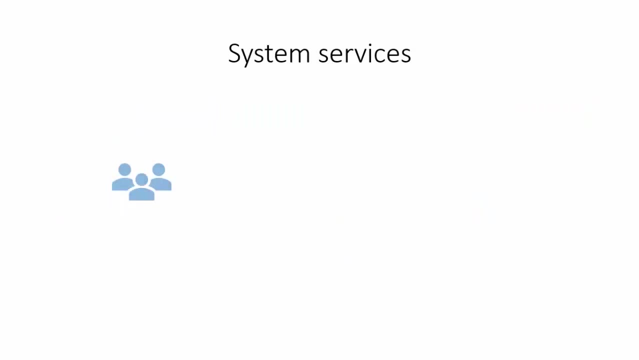 So these are the six services that an operating system provides to the user. Now the second set of services is for the system. So the operating system provides three services to the system. First one is resource allocation, Second is accounting And the third is protection and security. 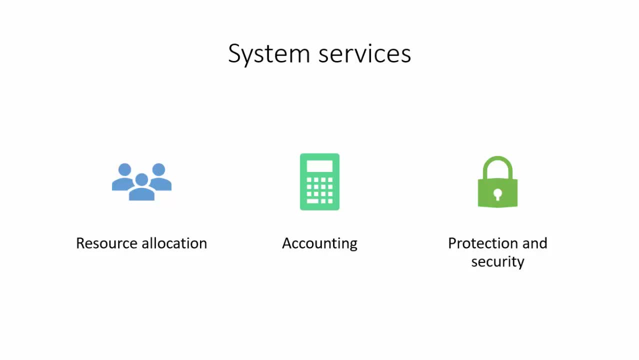 Now resource allocation. Since the system has got a lot of resources, the primary job of the OS is that it should allocate those resources among all the processes. There might be different processes which are running at the same time and they will be requesting for different resources. 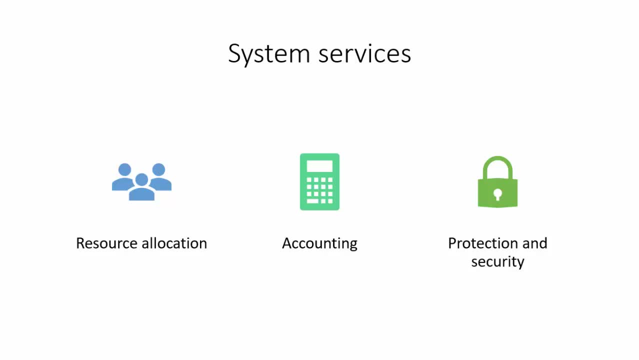 So the OS should manage those requests in such a manner that the request of every process is satisfied in minimum amount of time. The second service is accounting. Accounting means that the user should maintain track of all the users that are using the system. Let us suppose that as an admin, you want to monitor who all are using the system at what point of time. 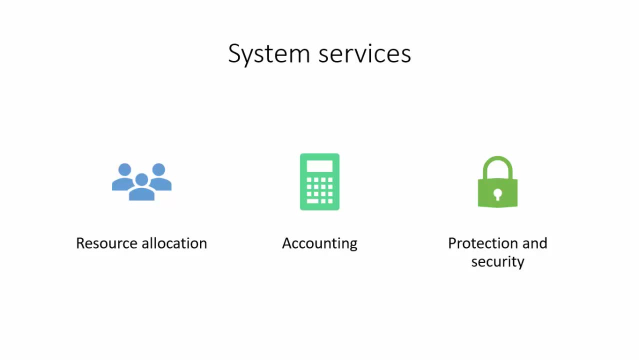 Then the OS has a service to offer in which you as an admin can create different accounts, One for each user. Whenever the user logs in, whatever activity he does, the OS keeps on recording that in a log file, And then, as admin, you can just go through a log file and see who has done what in what amount of time. 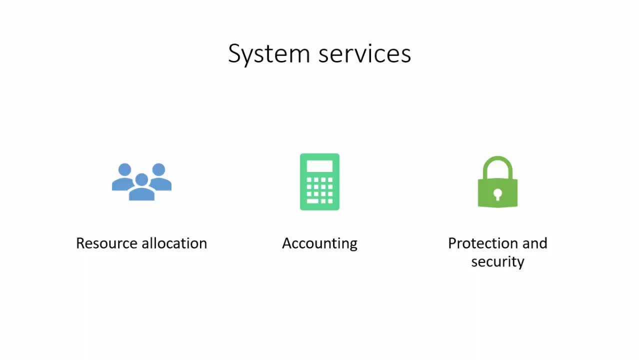 The last service offered to the system is protection and security. So protection means protecting the data from internal threats. Internal threats means protecting the data of one process from another process, Or protecting the data of one user from another user. Security means protecting the data from external threats. 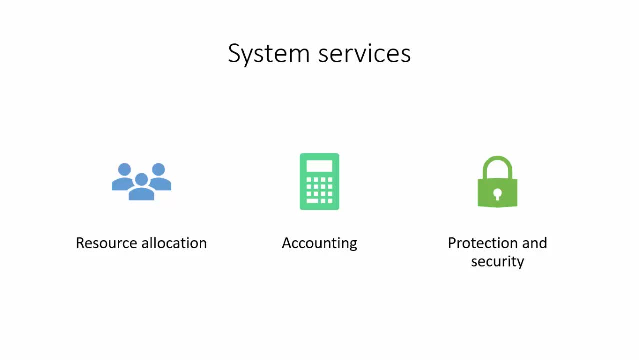 External threats can be what Virus, worms, etc. So there are different techniques used by the OS for that. One of the very popular techniques is using firewall. So these are the three services offered to the system. Now, in order to access any of the services, 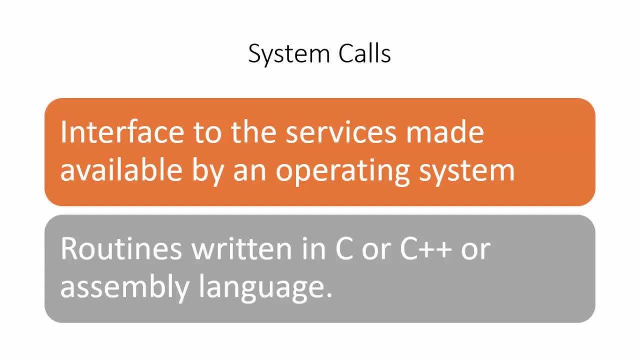 that we have just mentioned, you need to make use of something called as system call. System calls are routines written in C or C++ or in any assembly language. So in order to make use of the service, any service- you need to call the appropriate system. call for that service. 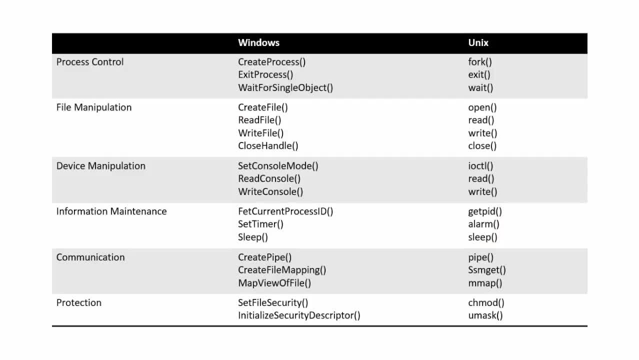 So this is a list of some system calls associated with the services that we have just mentioned. So the system calls are divided into Windows and for Unix, For example, if you want to create a process, then in Windows the corresponding system call will be create: process. 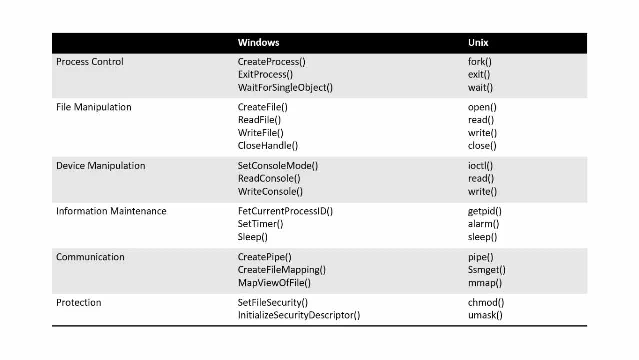 Whereas in Unix the corresponding system call will be fork. Similarly, if you want to manipulate a file, the system call for Windows will be create file, whereas for Unix will be open. If you want to read the file, the system call will be either read file or read. 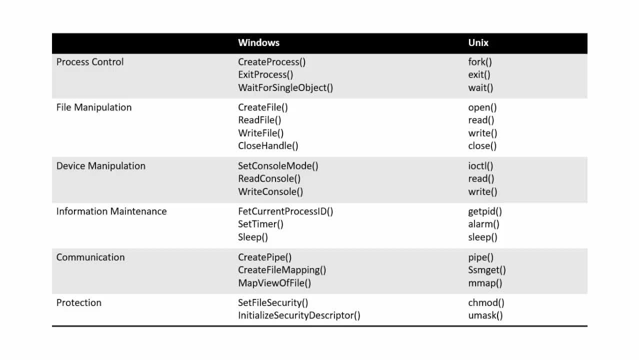 So you can just go through this. If you want to study them in detail, there is a separate series of videos on operating system lag in which we have discussed the system calls used in Unix. So on the same channel Dextrutor, you can find a list of lectures which are dedicated only to the lab part. 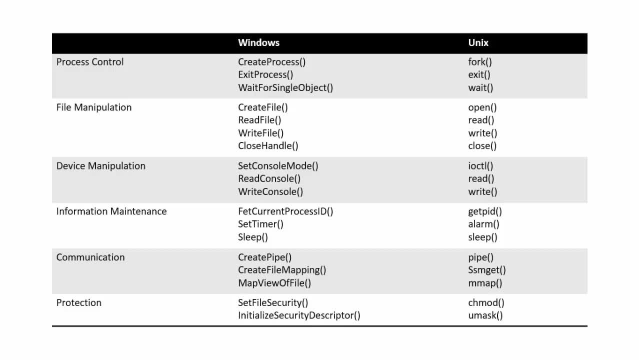 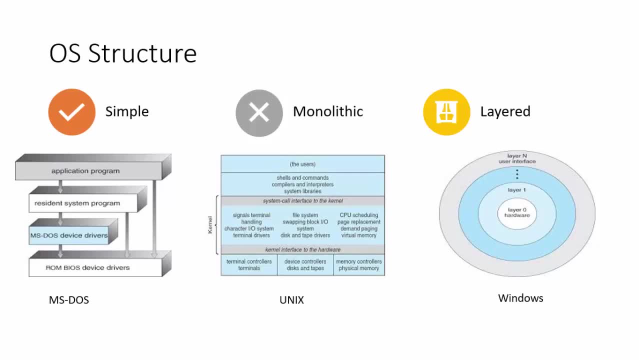 in which we have covered all the system calls in detail. Now, one last topic before we end up today's lecture is operating system structure, How these services are being handled in the operating system, How they are divided. So there are three structures. First one is simplest of the structure. 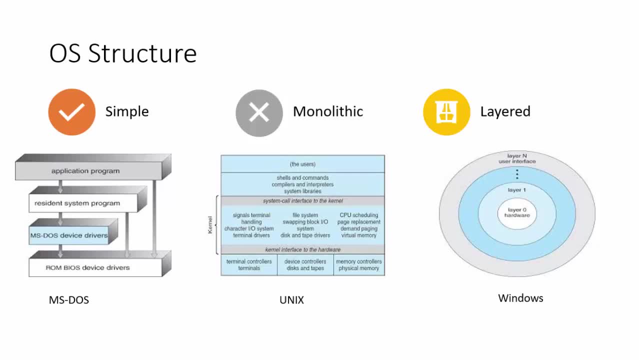 where the application programs can either pass through a layer of system programs, device drivers, and then they can go to the BIOS device drivers or access the hardware, or the application programs can directly access those hardware. It's a very simple structure, but this has a drawback. 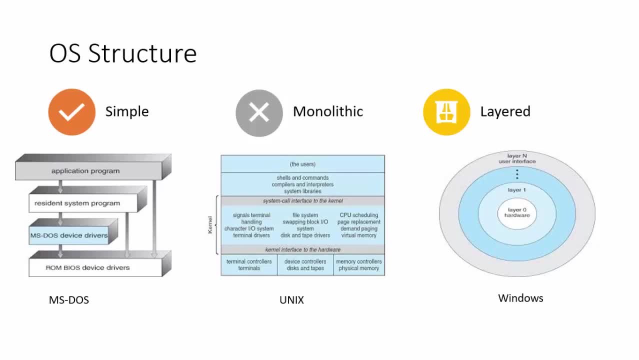 that the application program has a direct link to the hardware also. This means as a user, you can write a program which can directly access the hardware, which should not be allowed. A malicious program from a user or from a hacker can manipulate the hardware directly, thus damaging other user file or even damaging the operating system. 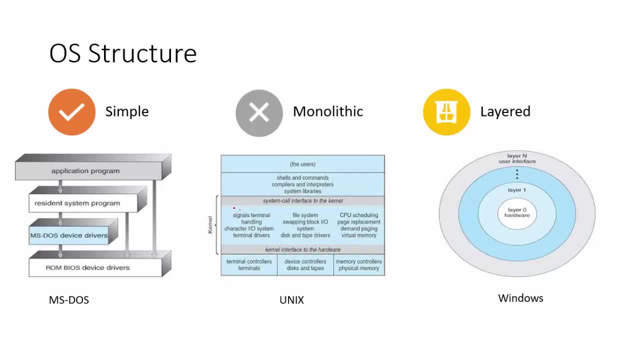 The second structure is a monolithic structure in which all the services are placed in a single function. This makes it very difficult one to code it and second to debug it also. So if there is a problem in one of the services, all the other services will also be stopped.